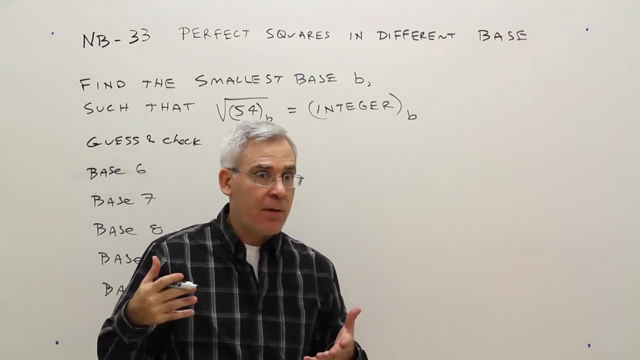 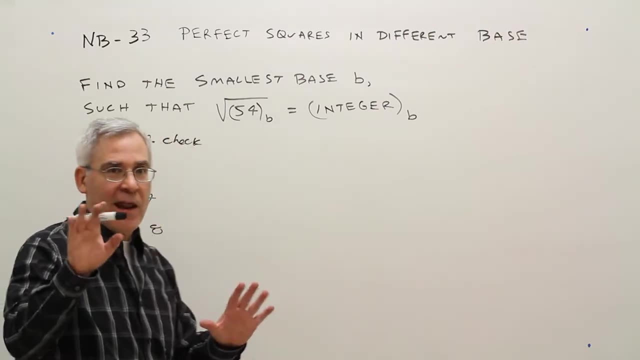 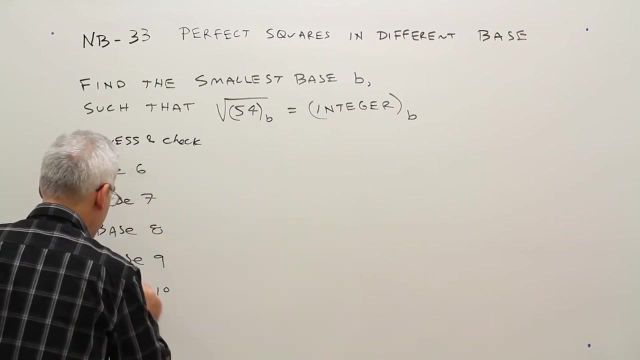 And for this unit, typically all the All the answers are between base 2 and base 16.. All right, so just to get a handle on it. in base 10, the square root of 54 is not an integer. 54 is not a perfect square, so just getting that out of the way. 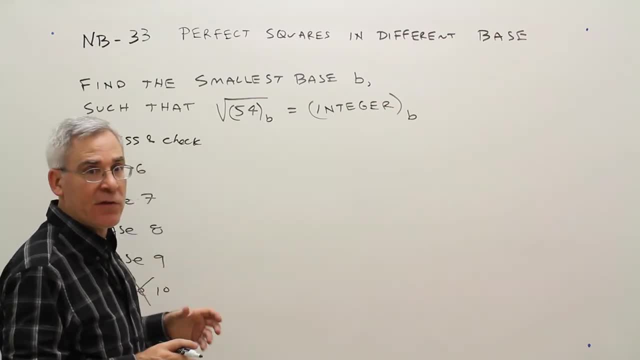 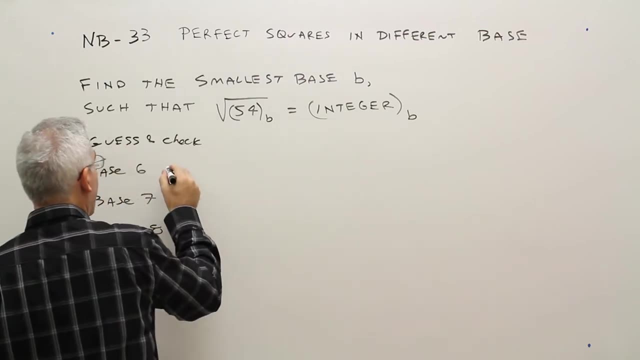 Okay, so let's go to base 6.. So if this were base 6, let's expand it to base 10, because I'm really good with my perfect squares in base 10.. All right, so going to base 10.. 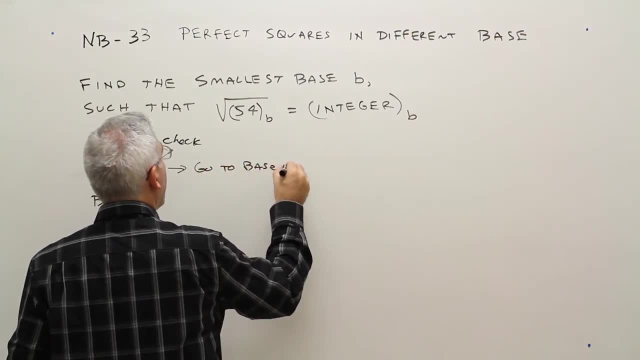 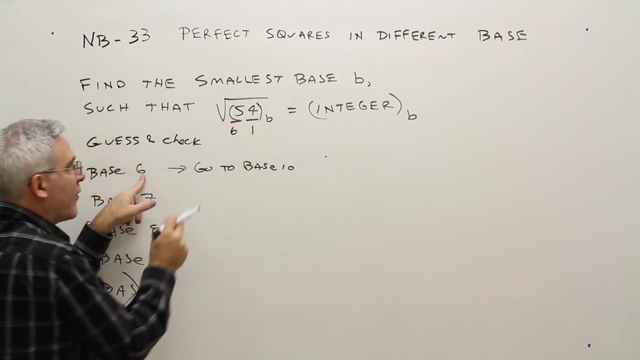 So go to base 10.. So this would be the, That's always the 1s and that'll be the 6s, And then over here will be the 1s and the 7s, the 1s and the 8s, etc. 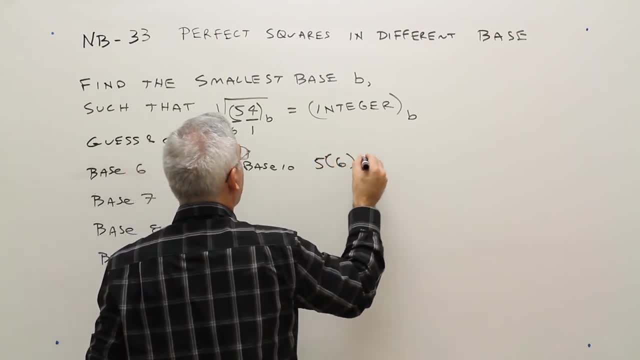 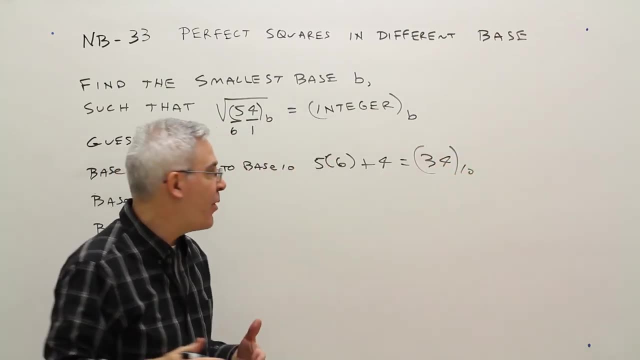 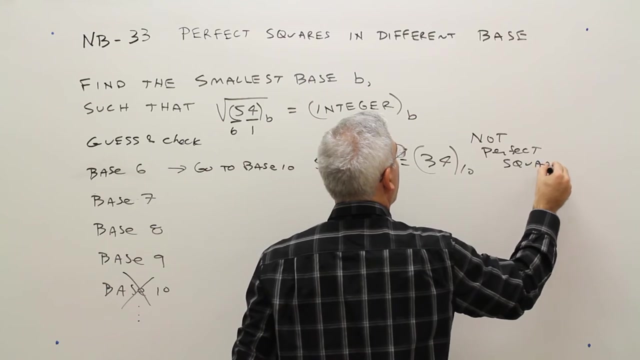 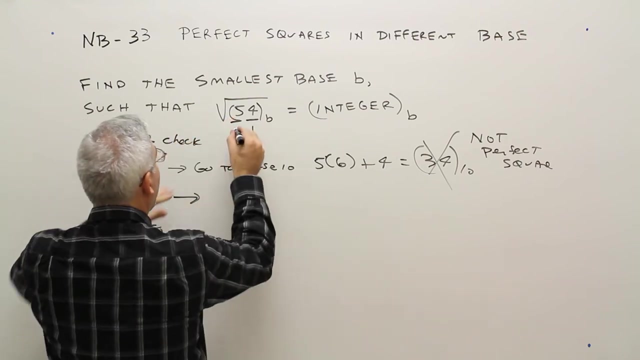 So over here it would be 5, 6s plus 4.. That's 34 in base 10.. That's not a perfect square, So I cross it off my list. Let's try base 7.. Okay, so if it was base 7, then I've got 5, 7s plus 4 1s. 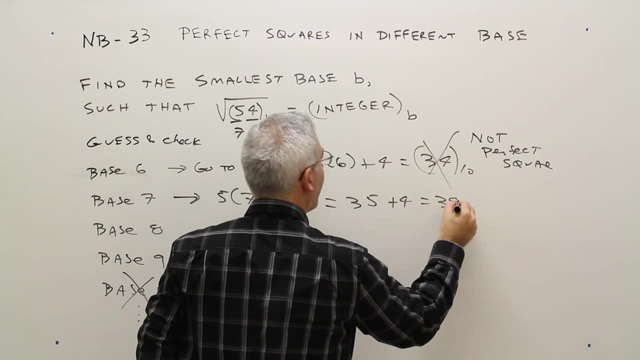 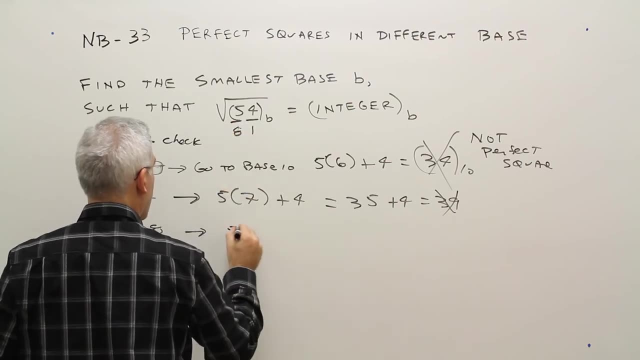 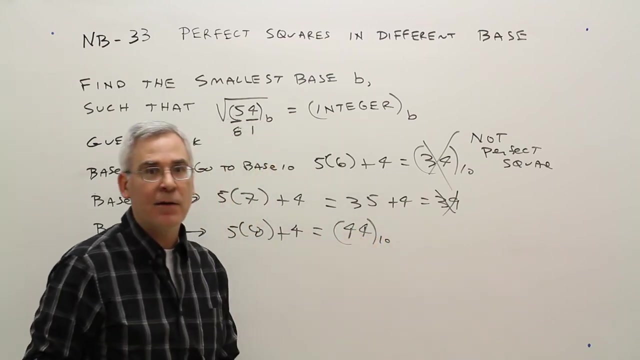 That's 35 plus 4.. That's 39.. Not a perfect square. Okay, let's try base 8.. 5, 8s plus 4.. That's 44.. That's 44.. And base 10, not a perfect square. 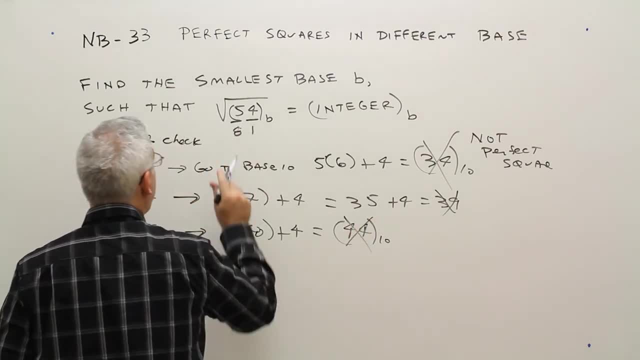 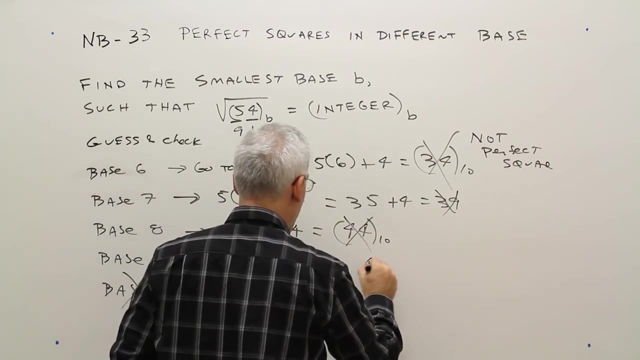 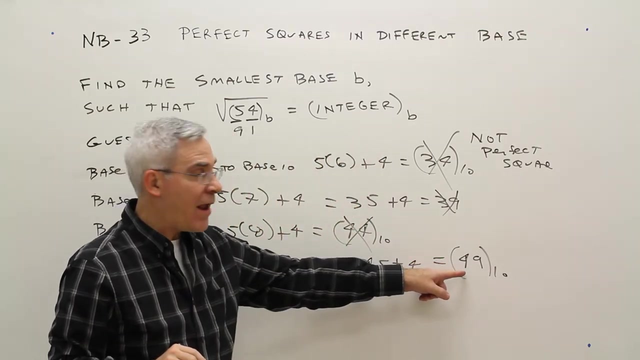 Oh, it's getting tedious. I hope this works out. Base 9.. 5 times 9 plus 4.. That's 45 plus 4.. That's 49 base 10.. 49 base 10 is a perfect square. 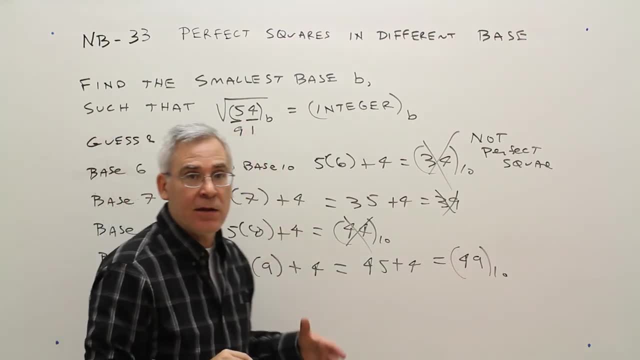 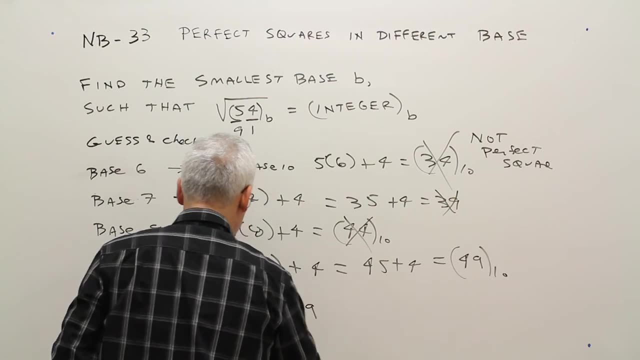 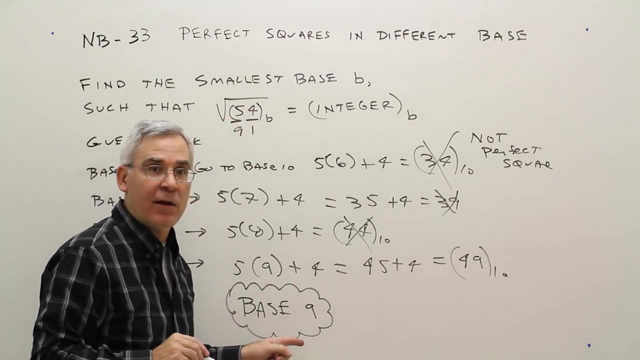 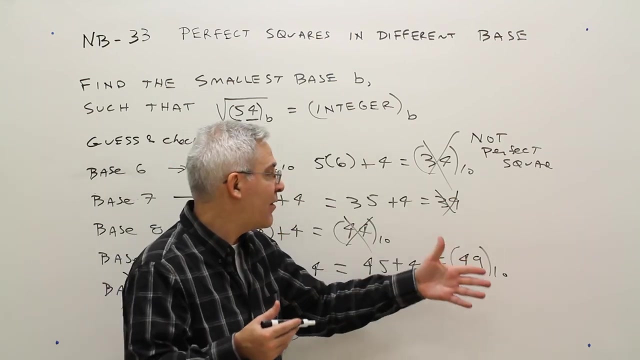 So that means that in base 9, this would work out. So again, 5: 4 base 9 is the equivalent of 49 base 10.. And the square root of 49 in base 10 is 7,, which is an integer.